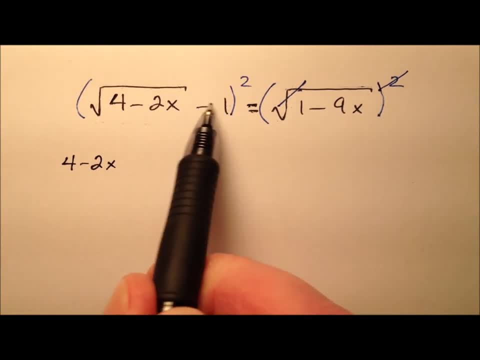 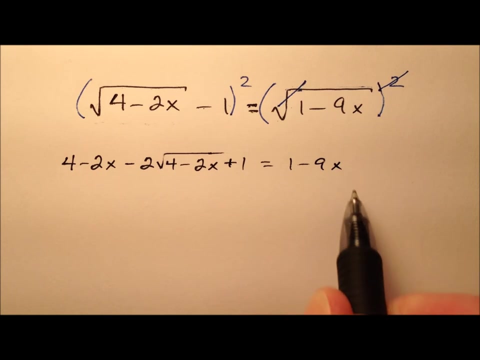 square root, Then we're going to go double the product of the two, So it's negative one times this, but we're going to double that, so minus two, And so that's what we'll have, And then the last one squared, so plus one, And that will equal now the one minus nine, x, And I will say this multiplication. 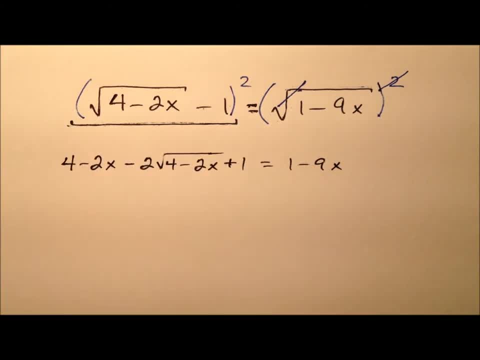 right. here is the single most common place that students make mistakes, So be very careful as you square this expression over here. If you have to put them side by side and not use a formula, then that's perfectly fine as well. Okay, so now we only have a single radical left, So let's go ahead and do a few things. 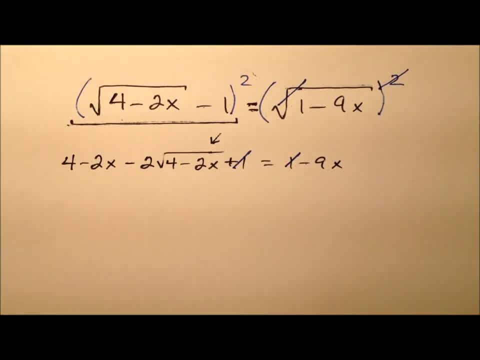 And notice that I have this positive one, positive one, so I can automatically cancel those out. And let's subtract four and add two x to both sides. So we'll subtract four and add two x, And again. this is in an effort to get that second square root of the two. So we're going to do this. 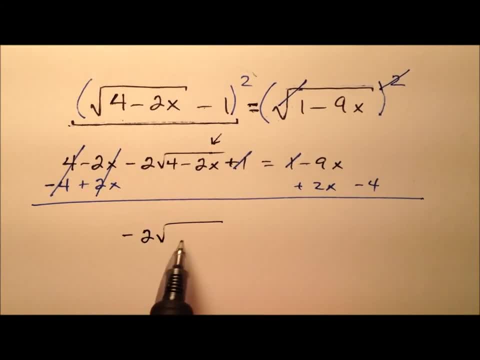 expression isolated. So we have the negative two times the square root of four minus two x, And that's going to equal negative seven x minus four. Okay, a lot of negatives everywhere. So why don't we just go ahead and divide both sides by that negative, so we can cancel this negative? 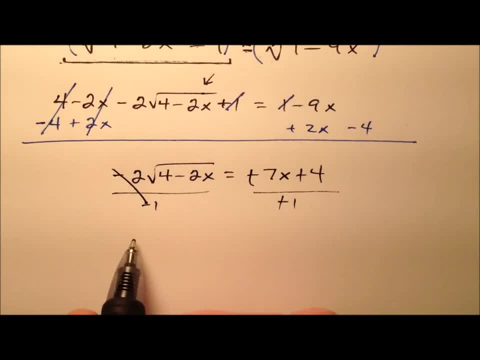 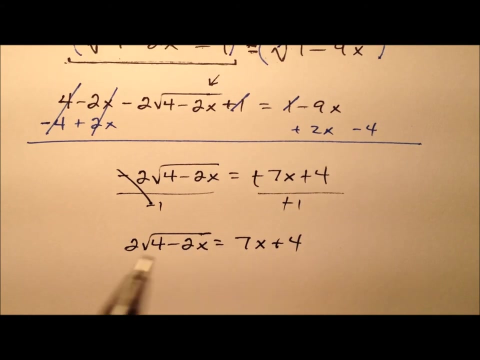 this negative and this negative as well, And that might be a little easier to work. I don't really know. We'll see how it turns out. Okay, so here's a consideration to make. We could really get this square root expression all by itself by dividing everything by two, But since these numbers, they're not both. 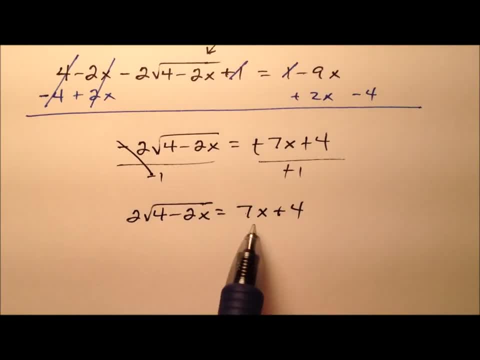 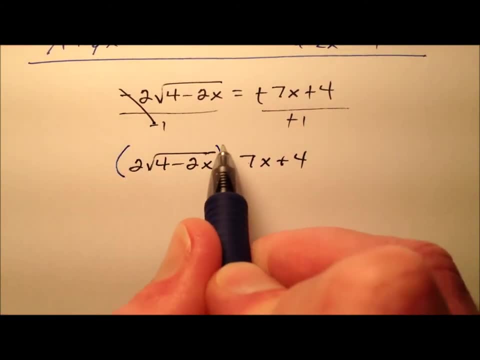 even I'm not sure dividing by two is the best course of action, because this would be seven halves x plus two And we're gonna have to square that. So maybe let's just go ahead and square it just the way that it is right here. So on this left side we'll square the two. 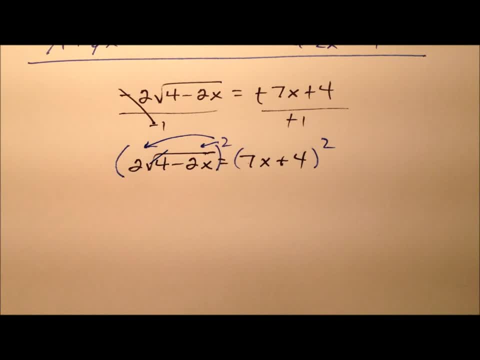 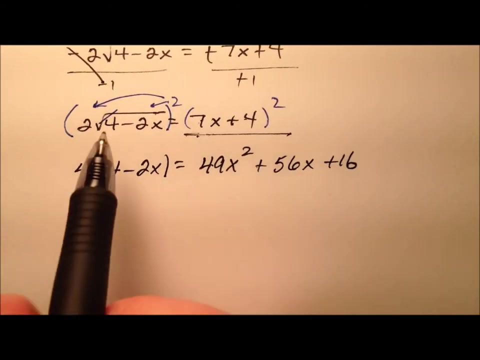 and we'll square this. well, square root expression. So we'll have four times four minus two x, And we're going to square this binomial So it'll be 49 x squared plus, and seven x times four is 28 x, but we have two of those, So 56 x and then plus 16.. All righty, so we'll distribute, So 16. 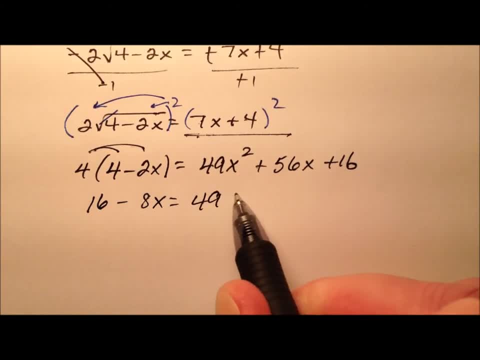 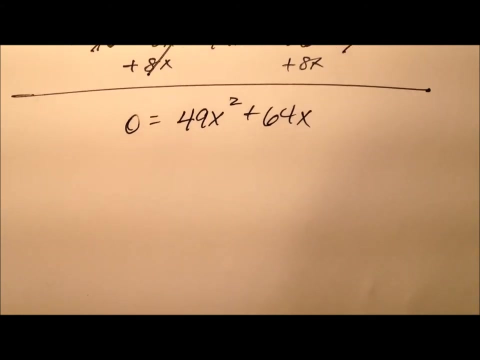 minus eight x equals 49 x squared plus 56 x plus 16.. Whew, this is actually not bad, because these 16s will cancel And we can add eight x to both sides And we'll have zero equals 49 x squared plus 64 x. Okay, this is not a bad place to be at all. 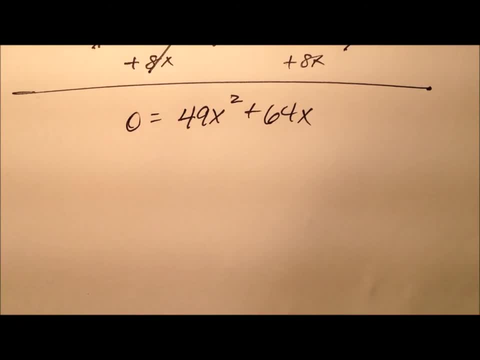 because we don't have to factor a trinomial. We're just going to factor this using the greatest common factor, which just looks like x. So pull that x out, So we'll have 49, x plus 64. And we have these two. 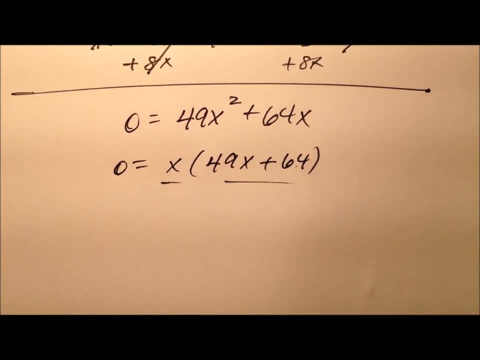 factors. They're being multiplied together to give us this zero. So we're going to use this zero property of multiplication and we're going to set both of the factors equal to zero. Well, this first one is really nice because, well, x equals zero. The second one, not quite as nice. 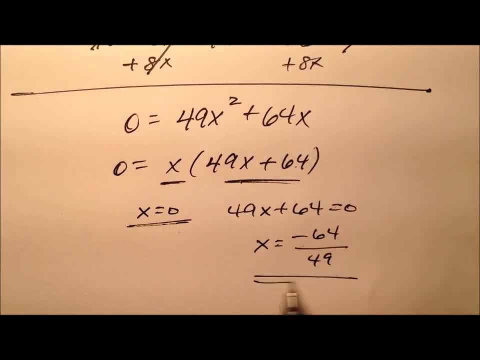 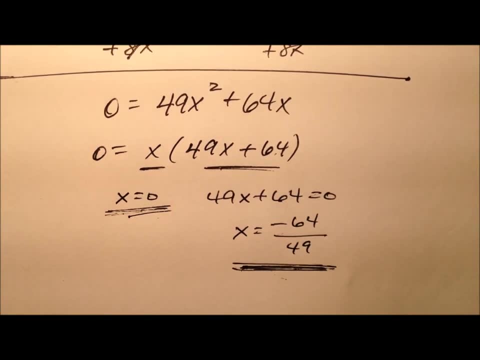 We'll have: x equals negative 64.. Over 49.. So one value is really nice and one value is kind of an awful-looking fraction, but that's okay. But remember, we need to plug these values back into the original equation to ensure that they work and they're not extraneous solutions. 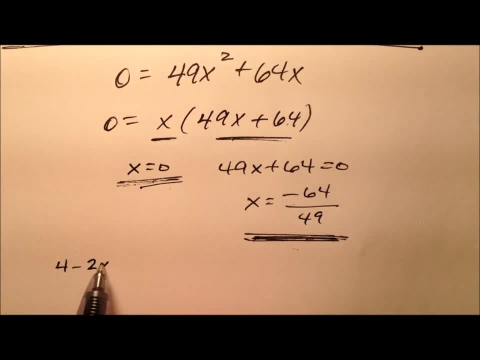 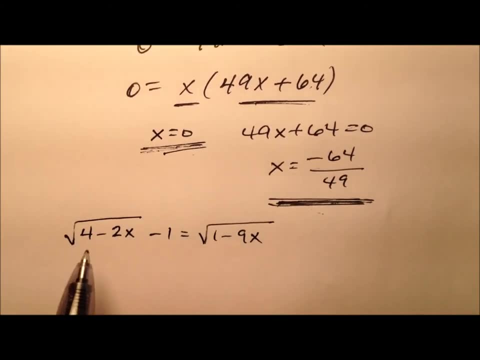 So let's go ahead and I'm going to rewrite this original equation. So we had the square root minus 1, equaling this square root, And let's plug in zero first, So it looks like 4 minus 0.. Well, that'll just be the square root of 4 minus 1.. And if that's zero? 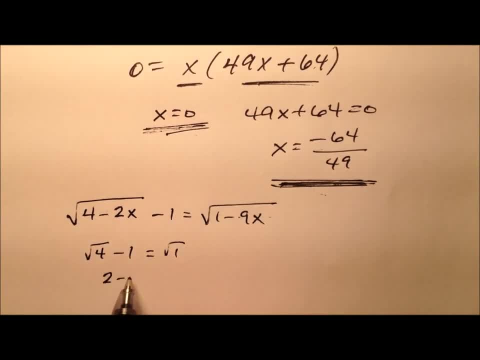 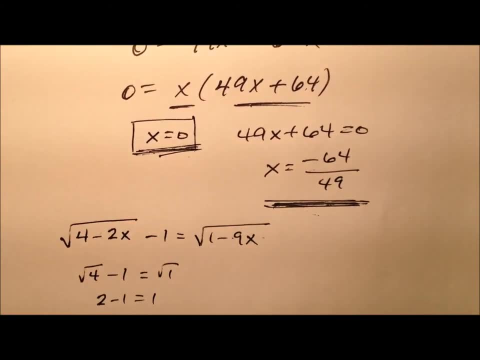 that'll just be the square root of 1.. So it looks like 2 minus 1 equals 1.. 1 equals 1. And I like that. That's nice. So we know that this x equals 0 works All righty, So let's go ahead and try. 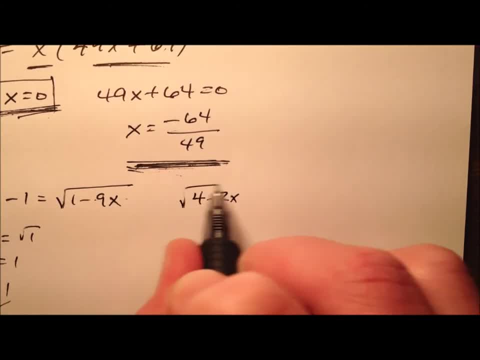 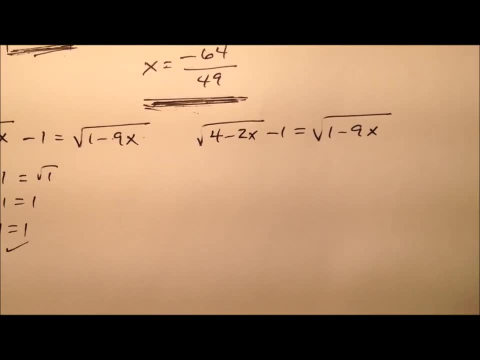 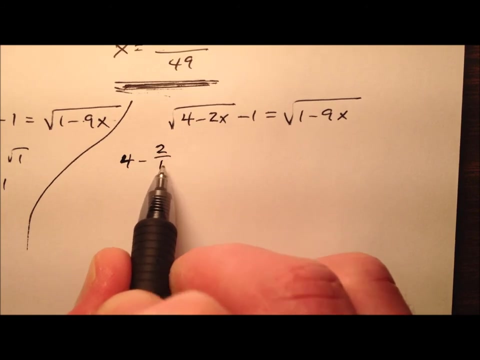 this fraction here. So I will one more time rewrite this original equation and we will plug this next negative 64, 49ths in. Okay, So make some room here. So 4 minus, we'll say 2 over 1 times negative. 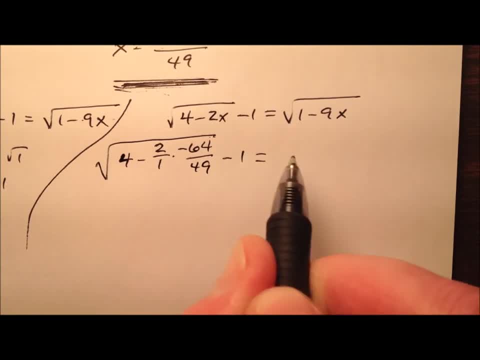 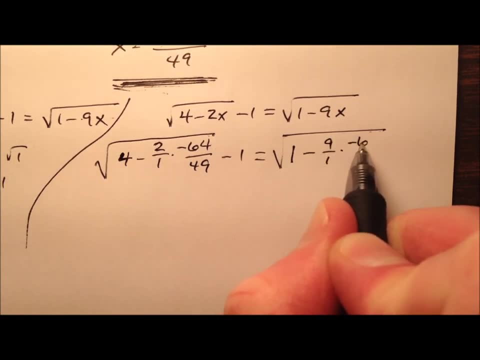 64 over 49.. That's all under the square root equals. let's see: minus 1 equals this square root here. So 1 minus 9 over 1 times negative, 64 over 49.. Whew, Okay, Got our work cut out for us. 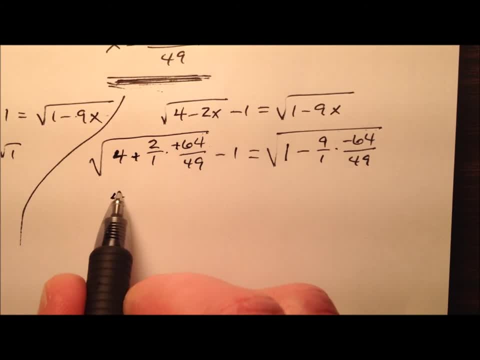 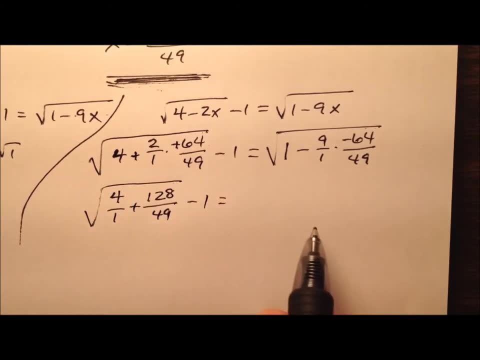 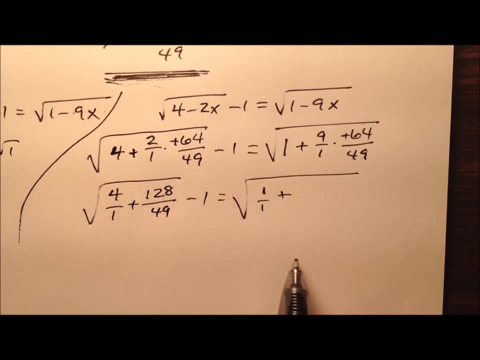 So the two negatives cancel. So it looks like I have 4 over 1 plus 128 over 49.. That'll be under the radical minus 1 equals And under this one these negatives will cancel. So 1 over 1 plus and let's see 9 times 64 should. 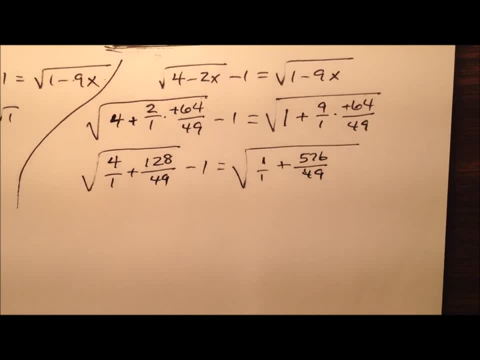 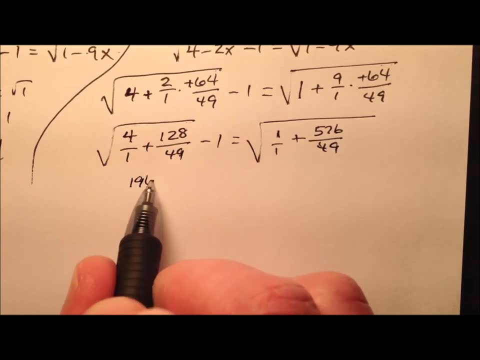 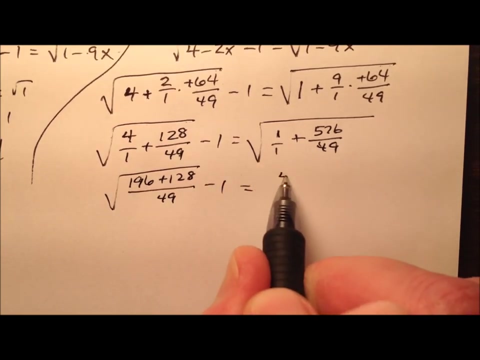 be 576 over 49.. Okay, So let's get common denominators for everything. So 4 times 49 is 196. So 196. So 196 plus 128 all over 49. That's under the radical minus 1. So this will be 49 plus 576. 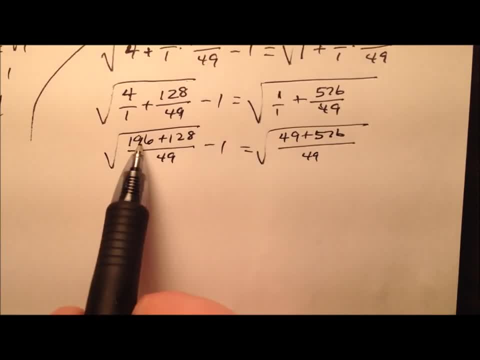 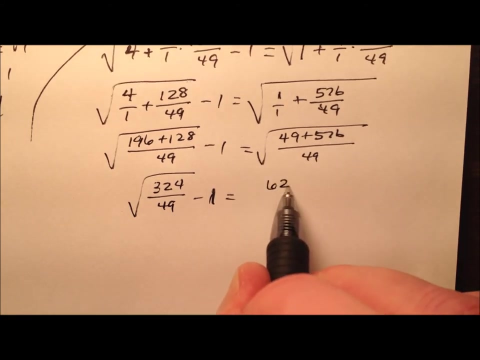 over 49.. And that's under the radical. So 196 plus 128 should come out to be 324.. And that is a perfect square, And 49 is a perfect square. Okay, Well, maybe this might come out nicely: 49 plus 576, that's 625.. That's a perfect square over that. 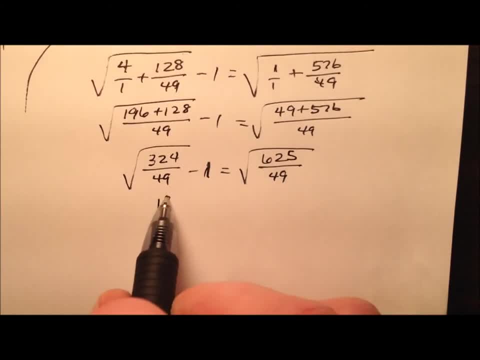 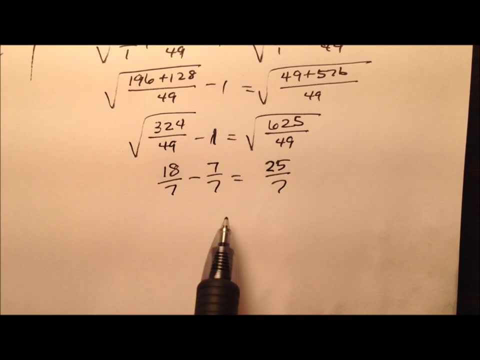 49.. That's a perfect square. Well, okay, So 18 sevenths minus 1,, which will be 7 over 7, and 25 over 7.. Well, it almost works. If this had been a plus right here, then it would have worked. But 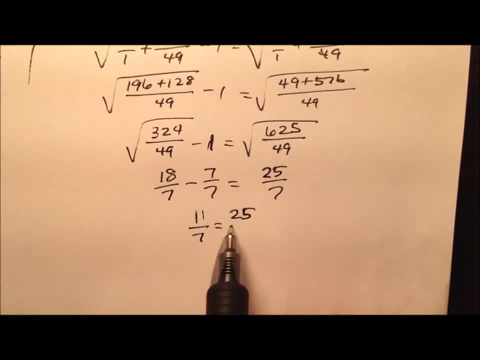 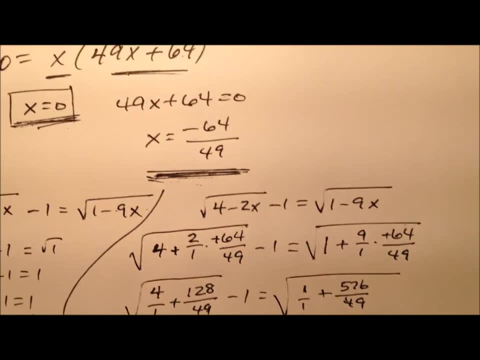 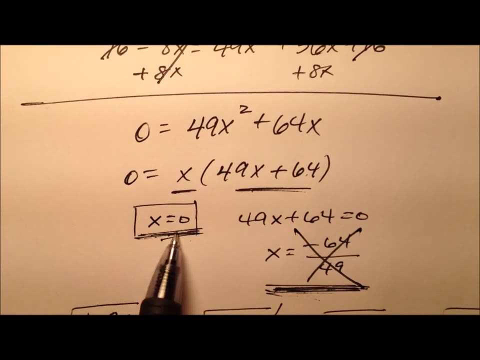 here we see: 11 over 7 equals 25 over 7.. And that's a no-go. So this negative 64 over 49 is going to be an extraneous solution. This will not work, So the only solution for this equation is going to be x equals 0.. And here was